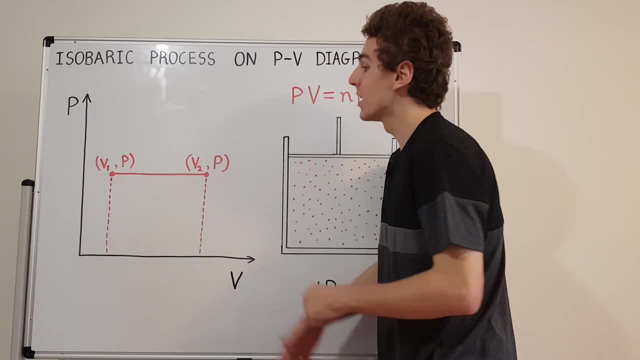 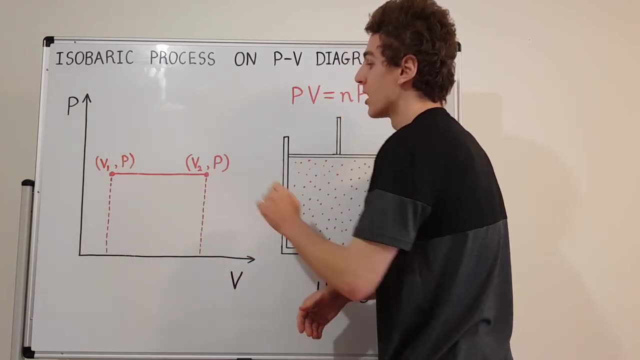 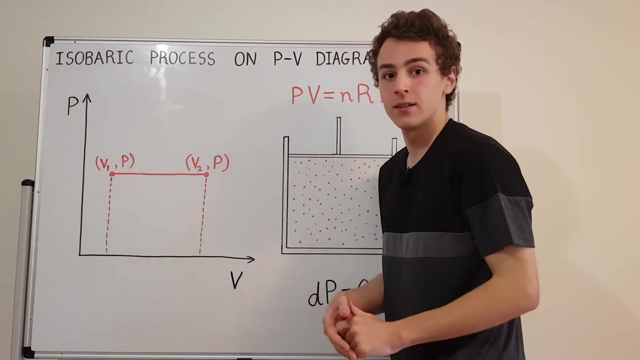 curve. So this rectangle over here is actually the work done in an isobaric process. These coordinates over here- v1p, v2p- correspond to the coordinates of the end and start points. Now what would happen if we started at v2 and finished at v1?? Well then we'd have compression. 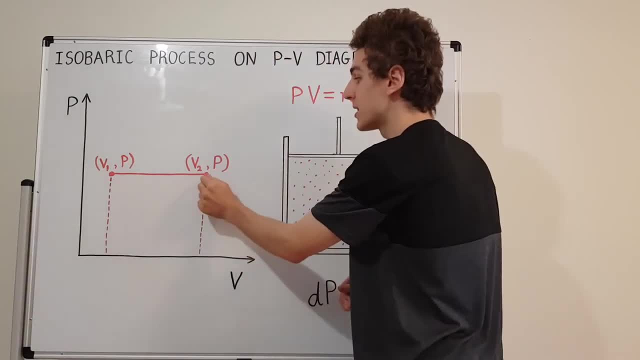 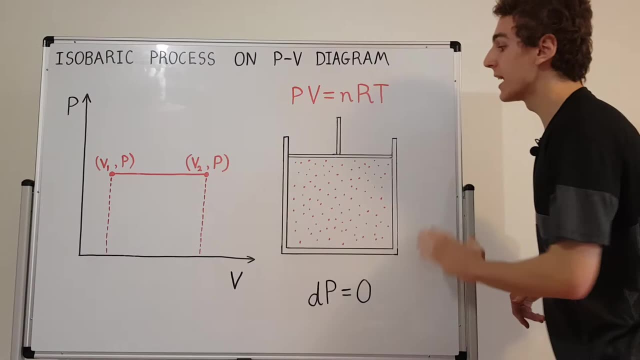 We'd be decreasing the volume, We'd be squeezing the gas. So in this diagram, we'd be moving along this horizontal line and we'd finish at this point over here. What would that look like in the actual physical real world? Well, that would be exactly the same as moving the piston down and compressing. 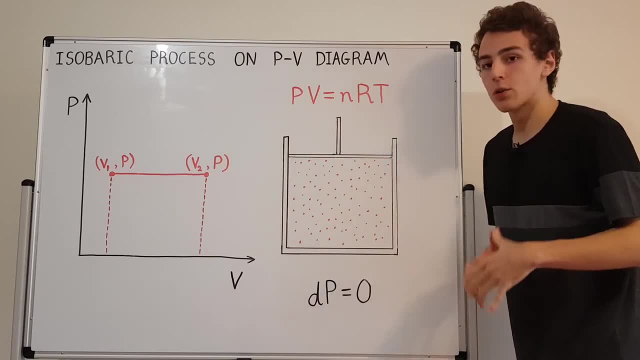 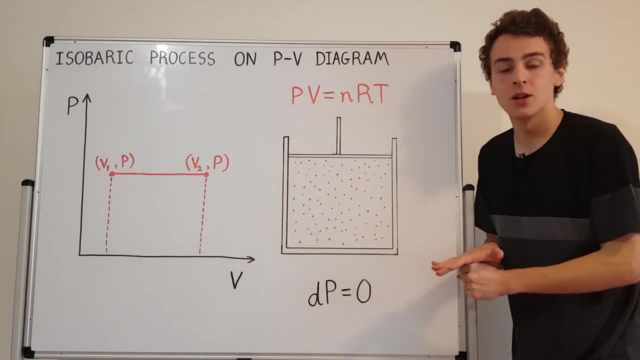 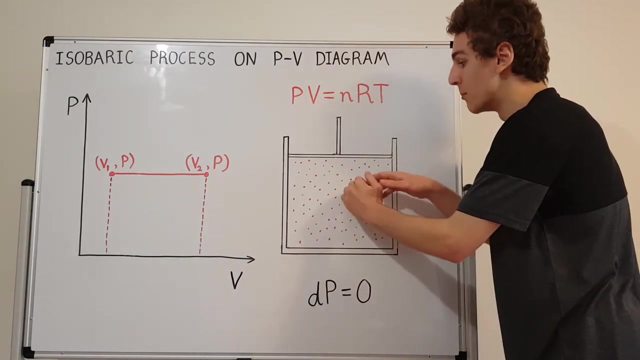 the gas. but if you think about this, you've got compression, but it's isobaric, which means it's constant pressure, so the pressure is not changing, but we're pushing down. so what is happening to that energy? well, it's actually being ejected in the form of heat. so heat is actually moving out. 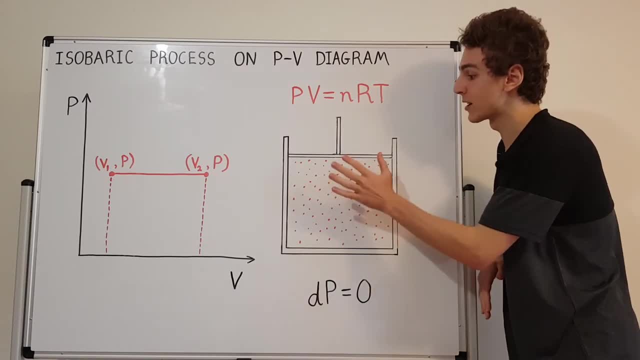 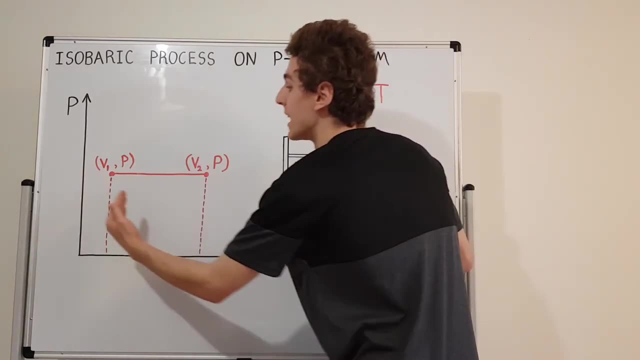 and the temperature is changing to adjust so that this remains at constant pressure. what if we did the opposite? what if we started at v1 and we moved up to v2? that would be expansion. so we start at this dot, we move along the horizontal line and we finish at this dot on the 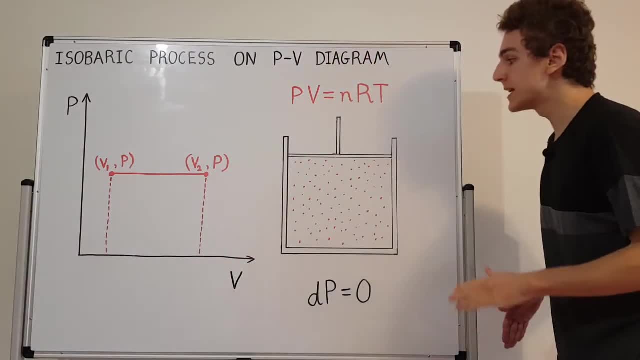 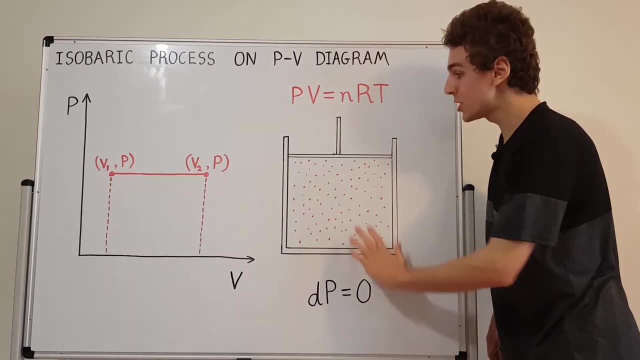 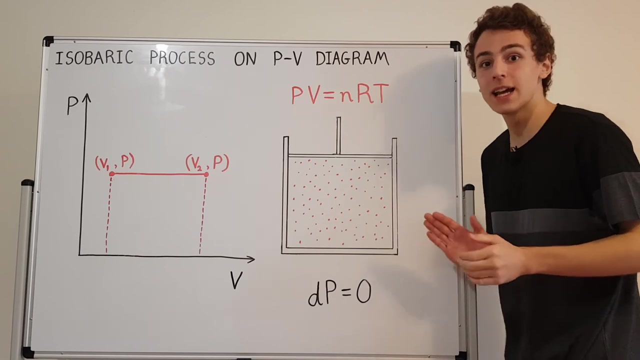 right. that expansion process would be exactly the same as moving this piston up. or, if you think about it, it's the gas pushing the piston up. so if the gas is pushing the piston up, then it needs to lose some energy. that work is negative. it's being lost to the surroundings because the gas is doing. 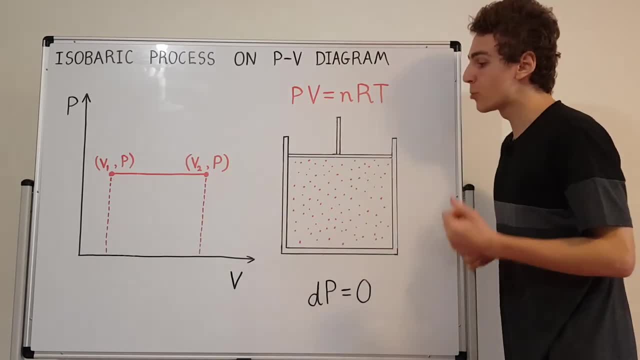 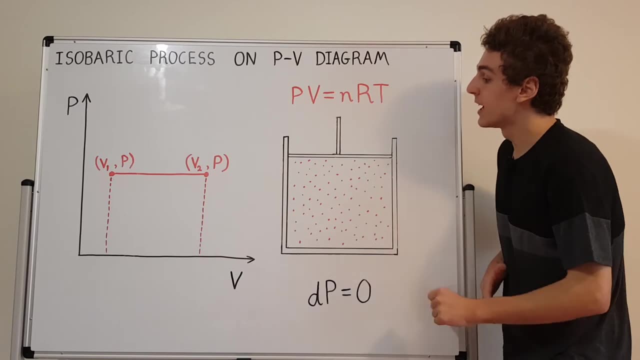 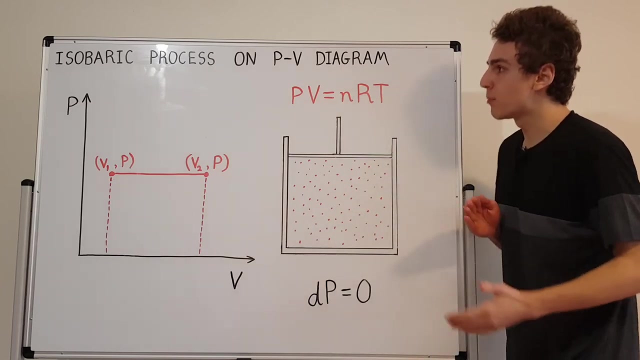 work on the surroundings by pushing the piston up. so where is that energy coming from? again, it's heat. so heat has to flow in, so the temperature changes in accordance with this ideal gas law and we have pressure remaining constant. so the important takeaway message for this video is that isobaric processes on the 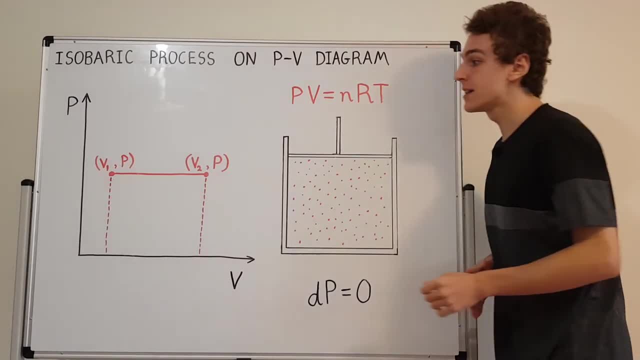 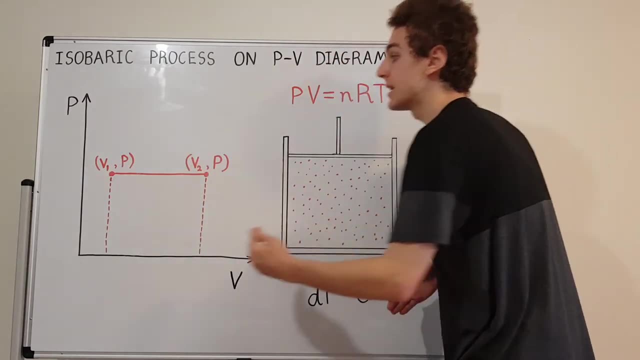 pv diagram are horizontal lines and the beginning and end points are the initial and the final conditions. if you move from left to right, that's the same as expansion. if you move from right to left, that's the same as expansion. if you move from left to right, that's the same as expansion.